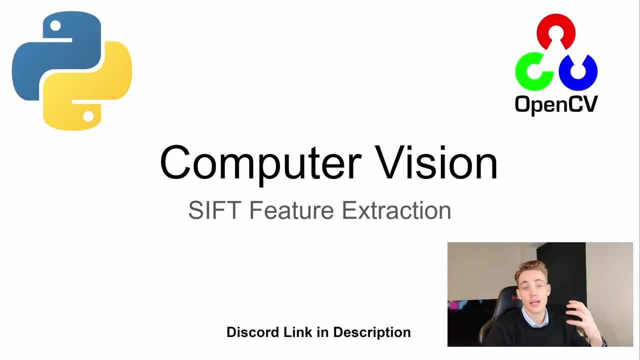 Then we can use SIFT feature extraction to actually get the exact points in both of the images. But first of all remember to join the Discord server. I'll link to it down in the description. here You can join the channel, chat with us about computer vision, deep learning, AI and so on. 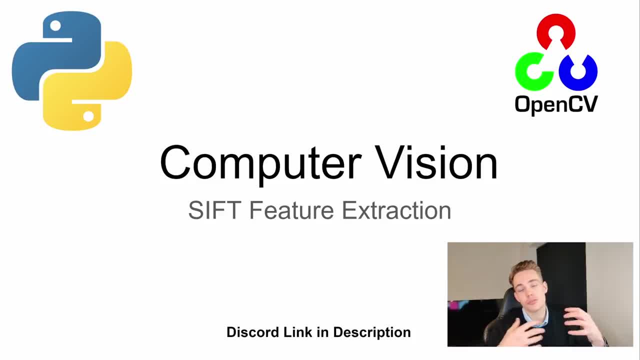 You can also become a member of the channel if you want to support the channel with a small amount of fee. Everything will go to create more and better quality content here on the channel. Also, if you're a member of the channel, I can help you out with some of your own problems in your own projects and applications. 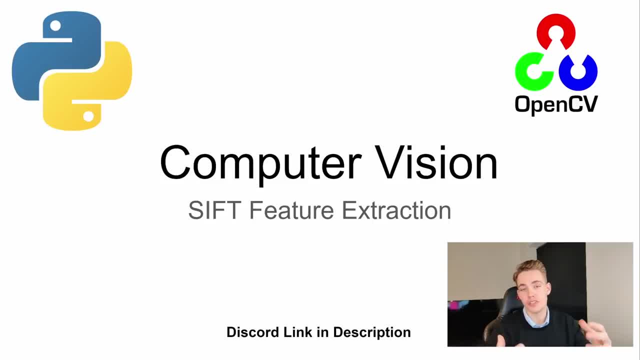 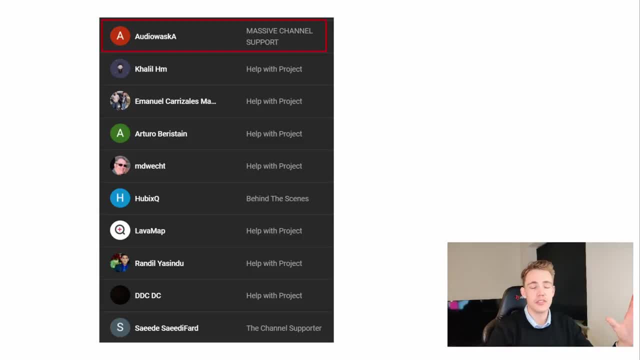 where I can guide you in the right directions and so on, if you're a member of the channel. so thank you guys. First of all, I just want to give you a massive shout out to these guys that are member of the channel. I'm helping some of these guys out here with some of their projects. 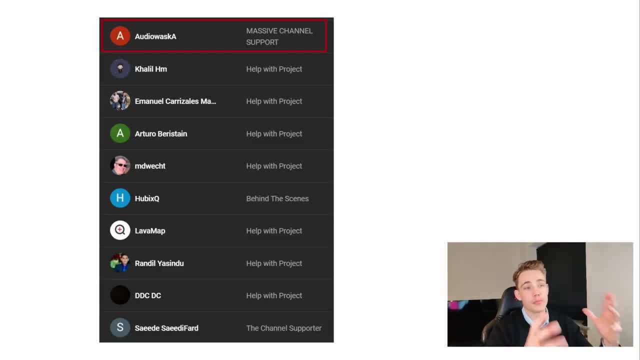 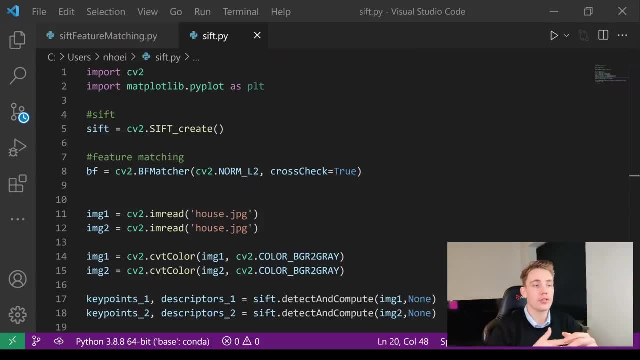 I'm guiding them in the right directions and so on. And also a special shout out to Audibasca here for the massive challenge report. I really appreciate it, guys. So we're going to go straight into the code here. I'm going to show you how we can set up the SIFT feature extractor here. 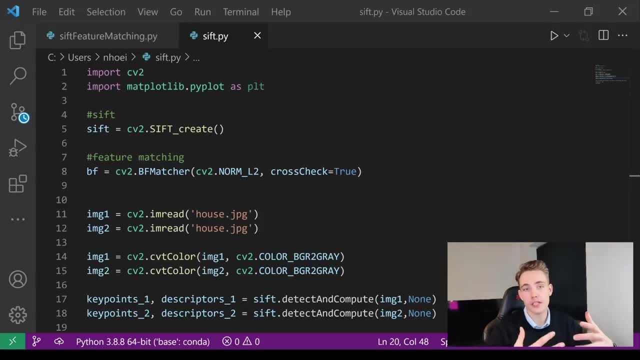 How we can match the different kind of features in the images and then how we can display it in the image. First of all, I'm going to show you a script here where we're just importing, or like reading, into images, So we're going to read in the same image and then we're just going to find correspondences. 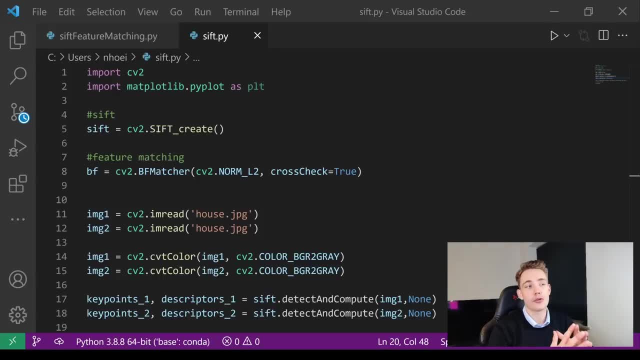 in those two images with the SIFT feature extractor And then I'm going to show you a script where we're actually going to open up the webcam and then we're going to load in the images from the webcam and then find features on live webcam feed of the environment or like me here in front of the webcam. 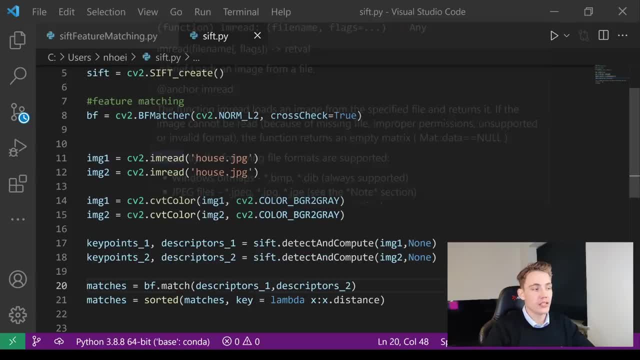 But first of all, again here, we're just going to take two images. We're going to read in the exact same image. So first of all, we need to import OpenCV. We don't need to import mapslib. We're not going to use that. 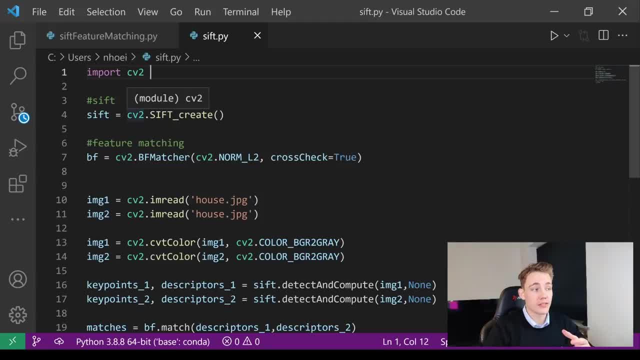 So we're just going to import OpenCV here, Then we're going to create the SIFT feature extractor. We just directly use OpenCV. So we just have the SIFT variable or object That we're going to create And then we have our modules- OpenCV module here. 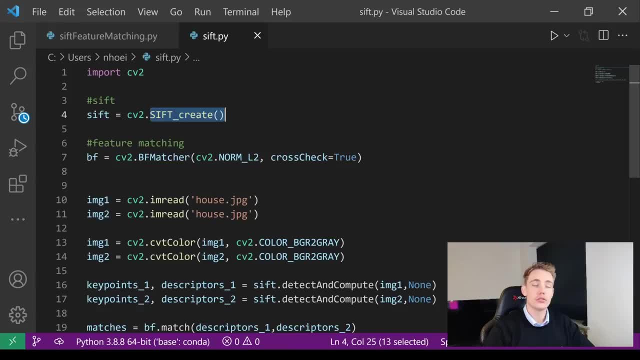 And then we can just call dot SIFT underscore create. So we just create this SIFT feature matcher algorithm, more like this class here that we just initialized, And then down here we also need to set up a feature matcher. So we need to define how we actually want to match the features that we're detecting. 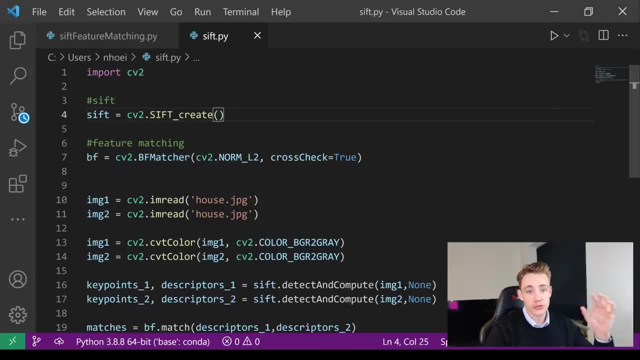 in the image with our SIFT feature extractor. So we're both extracting the features and then we're also matching the features from one image to the other image. So here Down here we're just creating our BF matcher here. So it's just a block matcher of different kind of like feature matches that we have. 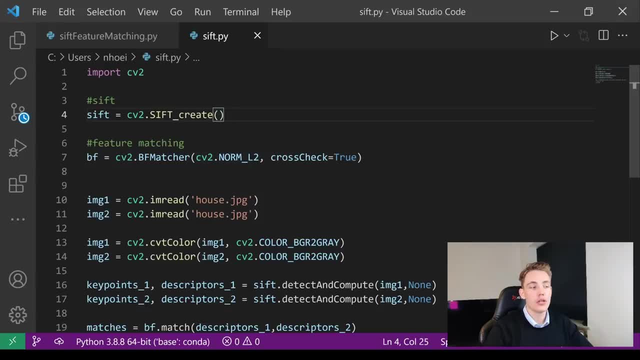 Then we use this normalization loss here, So we just use norm L2.. We can also use norm L1 here. It doesn't really matter, but you should use L1 or L2. if we're talking about SIFT feature extraction, We can also do cross check. 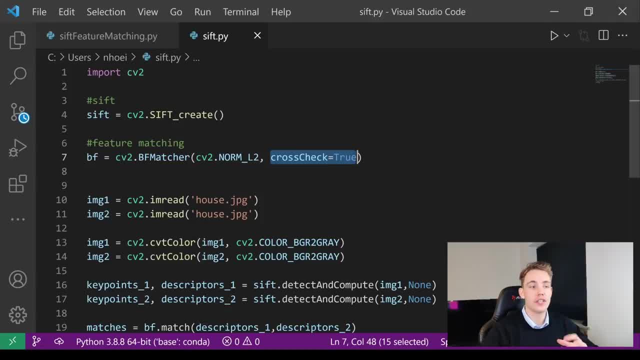 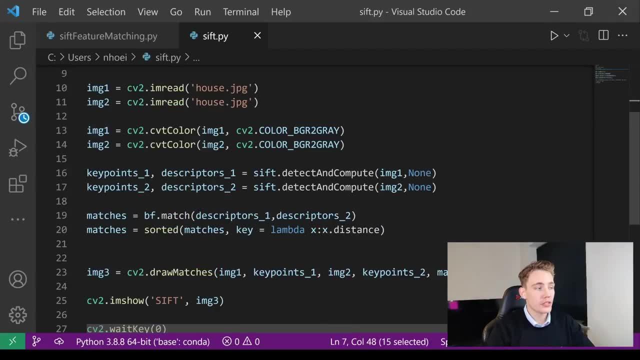 We can set that equal to true. Just if we want to do cross check off the different kind of points that we're actually matching or the features that we're matching in our image, Then we're going to read in the two images that we're going to do feature extraction. 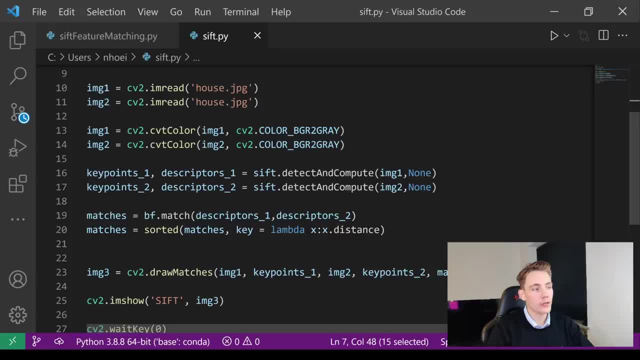 on. So we're just going to in read this house JPEG here, as we're going to see when I run the program. First of all, we need to convert our image from BGR image to a grayscale image, So we're only operating with one channel. 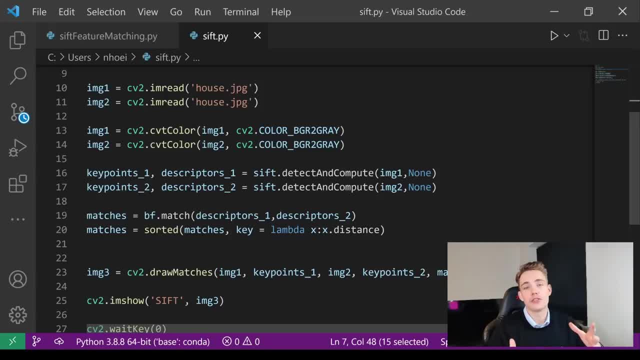 It will speed up the process and we're still able to detect all the features in our images. Then we'll get out the key points and also the different kind of descriptors that we can then match with our BF matcher or like our block matching, A algorithm that we set up here at the top. 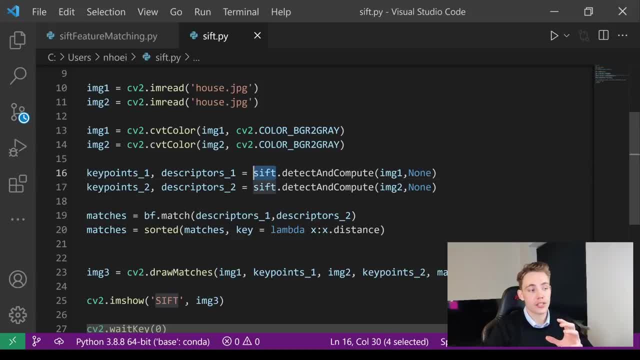 So here we're just going to call SIFT here. So this is our SIFT algorithm, or like a SIFT object that we created with this SIFT underscore create. Then we can just call dot, detect and compute. So we're actually just detecting all the different kind of features in our image. 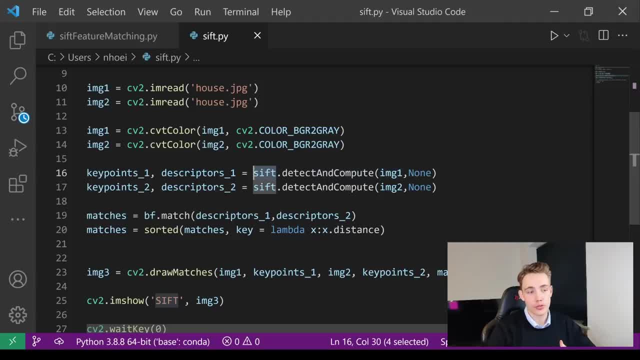 And then we're also computing both the key points and also descriptors here. Then we just pass in the image that we want to detect and compute the features in. We're going to do that for both images, of both in one and then two, and then we're going. 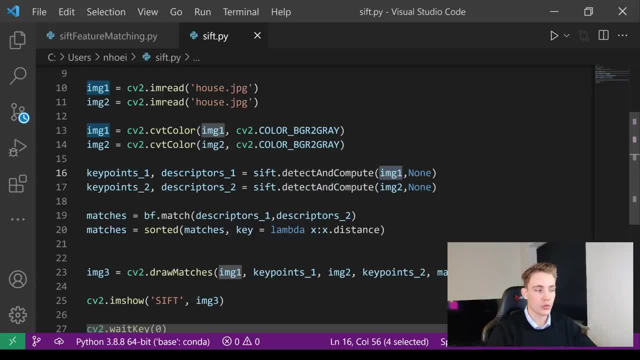 to store all information in the key points, one here, and the descriptors, one and the same, down here for our second image. So now we'll both get the key points in our images and we will also get the descriptors that we're going to match. So then we can actually go down here and create the matches with our BF block matching algorithm. 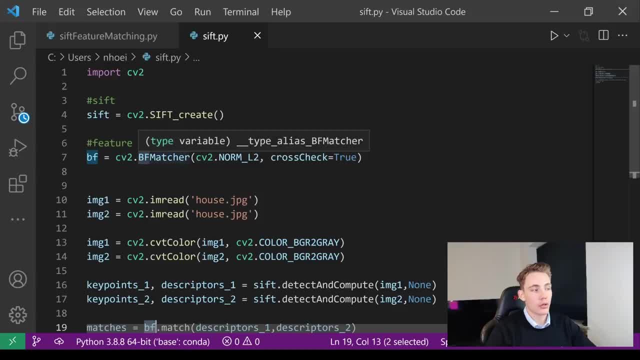 that was set up here at the top. So this will just be using this block, block, blocker, feature matching here, where we're just matching with this normal two loss and then we're doing cross check on our feature matching points. So we're going to just go in here passing the two descriptors that we actually want. 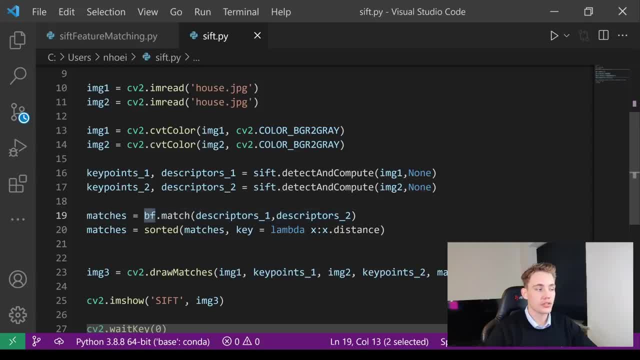 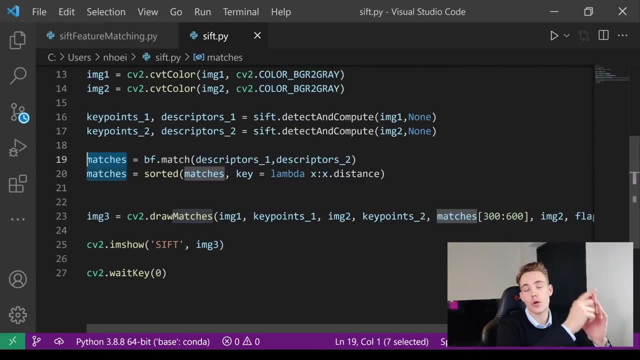 to match. We just call BF dot match, passing the two descriptors, and then we'll just get out this variable, which will contain all the matches that we have in our image. So a match is actually just one point that we're matching to another point in the other. 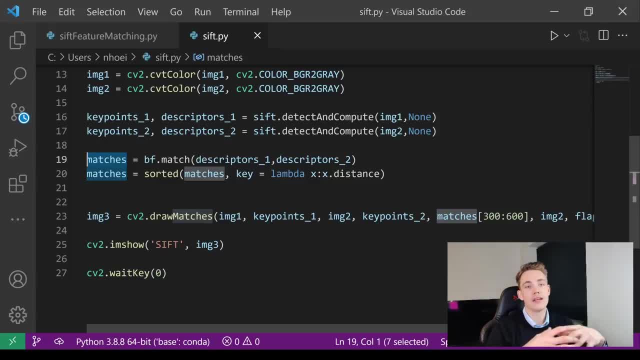 image that will. that will actually be a match and we want to display that in our image. It can be for a lot of different kind of things in stereo vision. if you want to find the exact same points that we want to match, For example, if you want to find the depth to an. 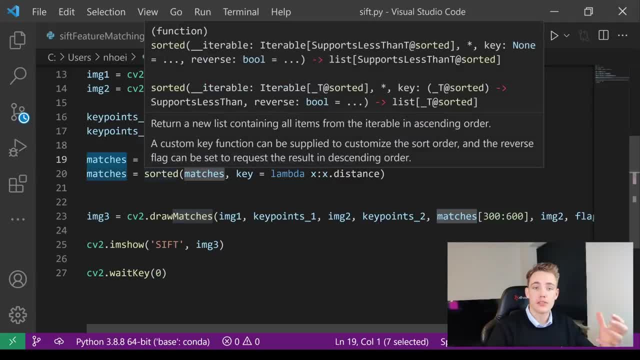 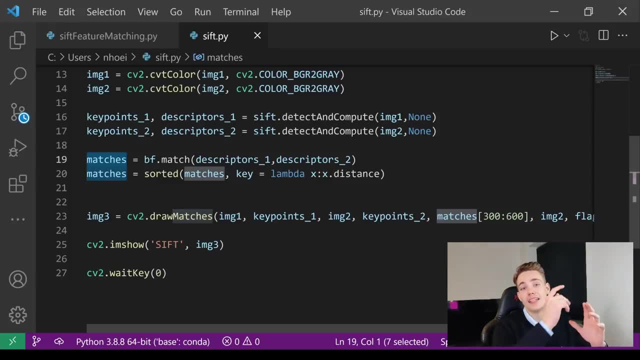 object in the image, then we can actually just use sift feature matching, feature extraction here or for some other different kind of approaches or methods or projects where you just want to find the exact same points in one image and another image. Also, if you want to rotate your points or like find the translation and rotation from 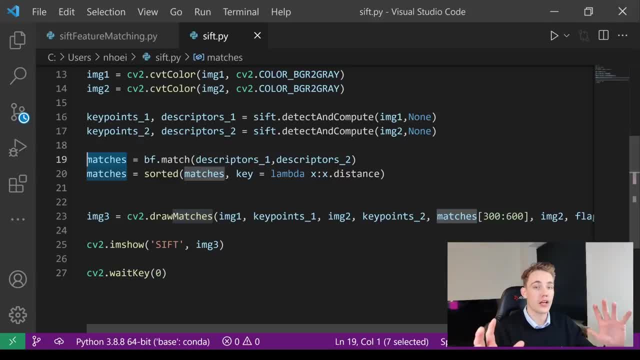 one image to the other and so on, So you can use for a lot of different kind of algorithms. and it's one of the hardest problems in computer vision is actually like to define how we're matching points in one image to another- The image- and finding the exact same points, even if the images actually look identical. 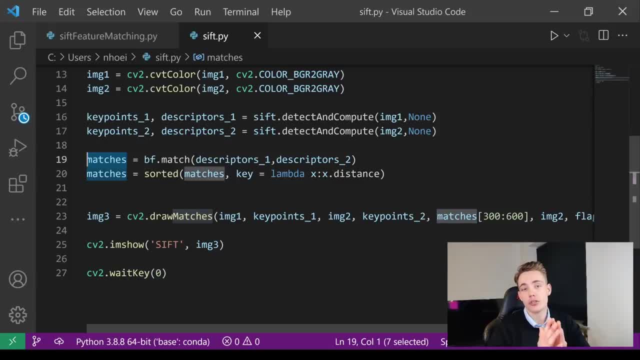 or like some of the different kind of corners in the images actually look identical. Let's say we have a background with one color, or we just like have a wall with a lot of windows or something like that, then a lot of the different kind of points in the image. 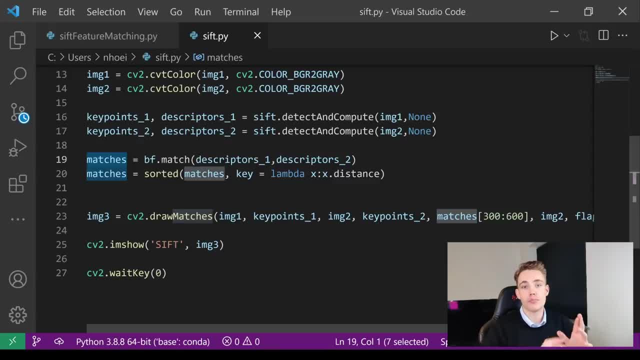 are actually similar, So that makes it really hard to match points from one image to the other image. But now we have all our key points, We have our descriptors and then we're matching our descriptors. All the information here will be stored in the matches. 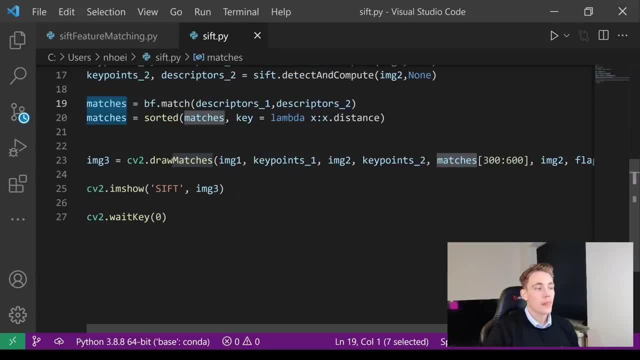 Then we can just go down, use OpenSV to actually like draw our matches. We just pass in the image the key points for the first image, second image and also the key points for a second image. So this would just be the key points that we actually like detecting. 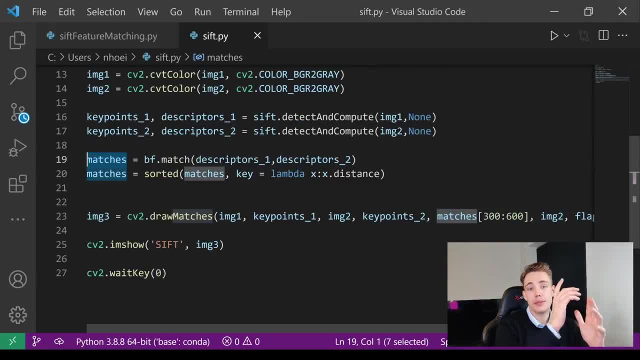 And then we just display our matches here, So the matches will actually be the lines from one point to the other point. So the key points, we have the points, which is the key points, And then we have our matches, which actually like the lines or like just the matches. 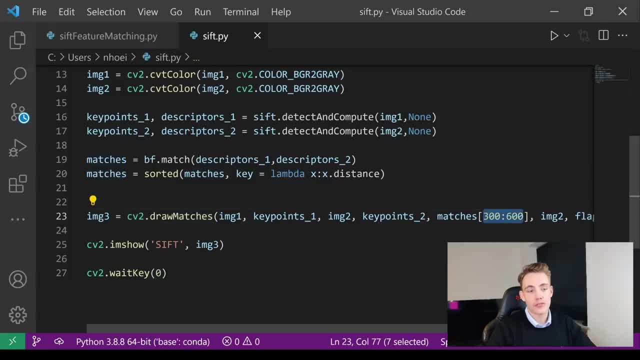 So we can just go down and just display the matches of those points together. We're just going to display the middle of the detected points here, because we're going to detect a lot of points in images and we can't display them all. Or at least we can see how we actually like matching one point from the first image to. 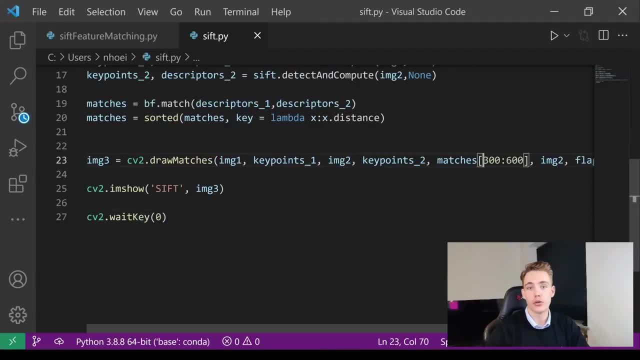 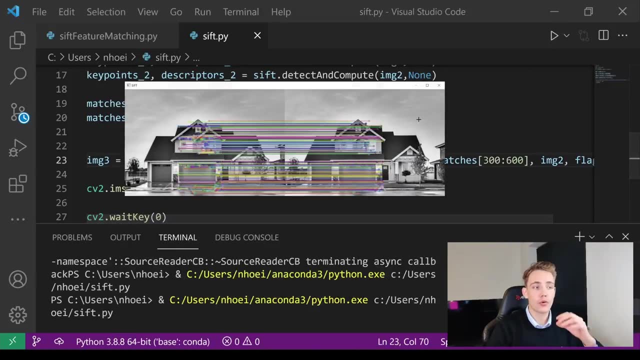 the second image. Then we're just going to show our SIFT results and we're just having this wakey here. So it'll just show the image until we hit a key on a keyboard and it will terminate the program. So let's now run it here. 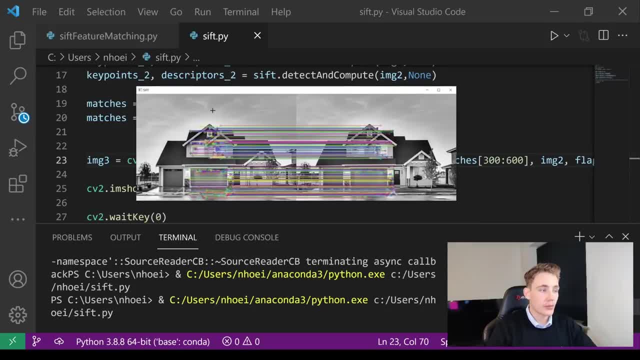 Before we're going out to open up the webcam feed. So now we get up the webcam feed After we get up the result. here we can see that we're detecting all the different kind of features or like points here in the left image. 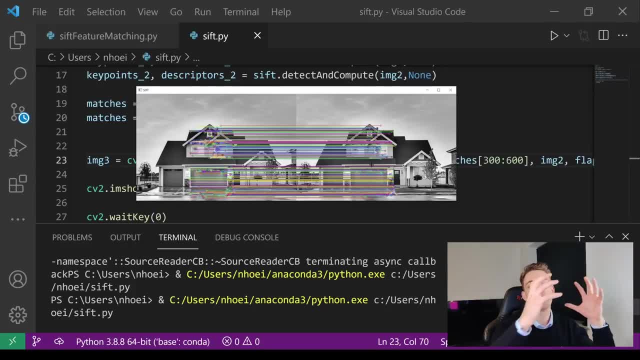 We're doing the exact same thing in the right image And then we're trying to match those points together. So we're trying to find the exact same points in both images. Again, as you can see, you can use this for stereo vision to get the exact depth of these. 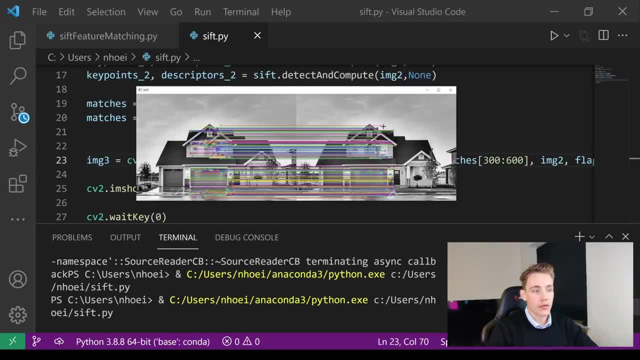 points as an example. But we see here, if you just take a couple of points like this point here out in the sky, it is actually like mapping this point here exactly to the same position here in the right image, Even though the background here there's not a lot of change here in the colors. 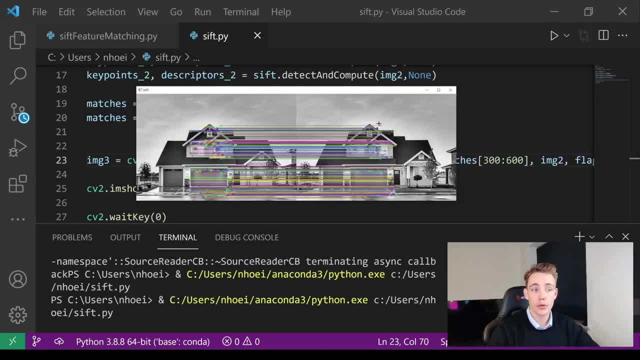 So this point could have been up here, here, here, here, but it actually matches this at the exact same location here, because this is actually a really good and really reliable and robust algorithm, this SIFT feature extractor. We can also take another image here or like another point. 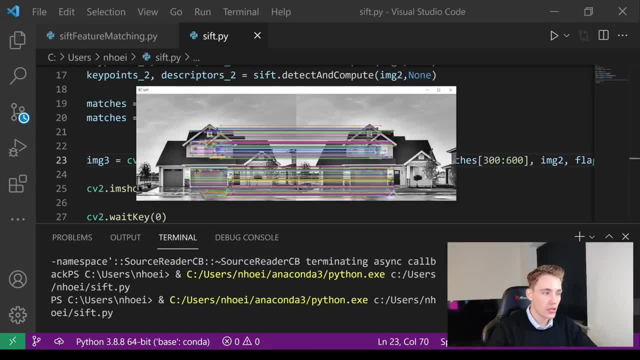 We can see the green one. here is the exact same point. We can go down here at the window. We can see some blue points here, actually like map to the same blue points Here. we see a blue point here, a blue point here and here. 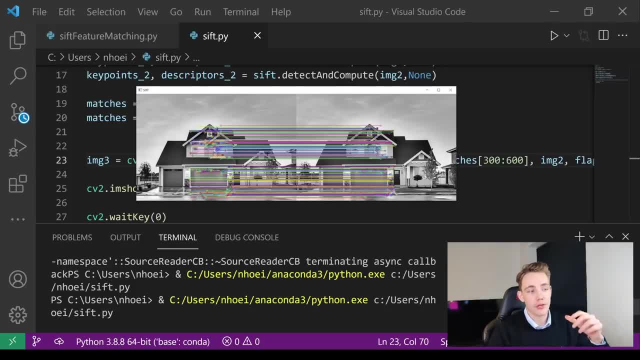 So we see all these points here is actually matching perfectly And we can also verify because we're using the same image. So all these lines here are actually like horizontal, because there's no change in the point here in the Y direction, or like in the right direction here in the image, because 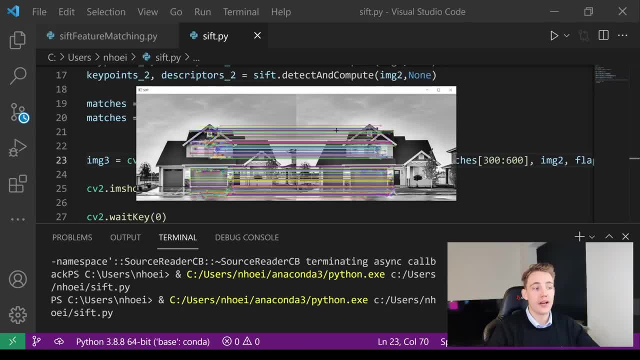 we're just taking two identical images, So if we find the exact same point here in the right image as in the left image, then there will be no change here in the image In the Y direction, which is why all these lines here are horizontal. 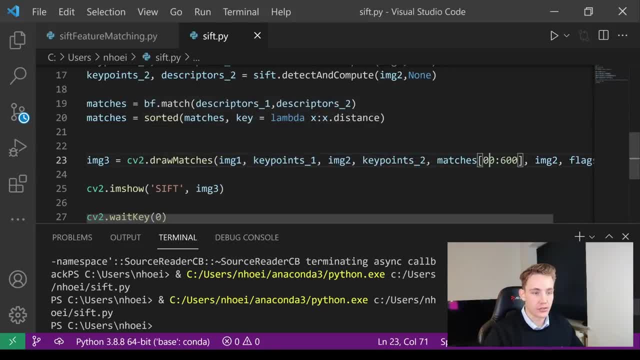 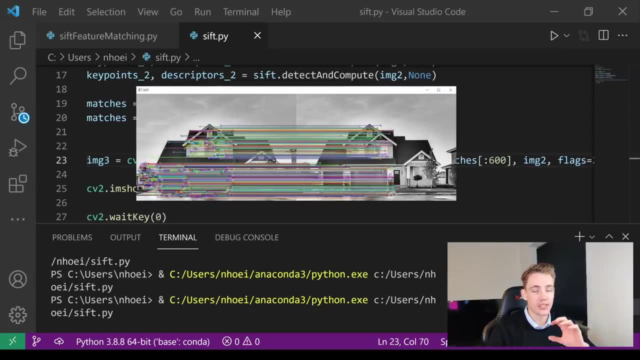 So this is really nice. We can. we can actually just try it here. We can just set it to zero or we can just take 600 points in our image and then we can see that we get all these points down here in the tree and we can see we find a lot of. 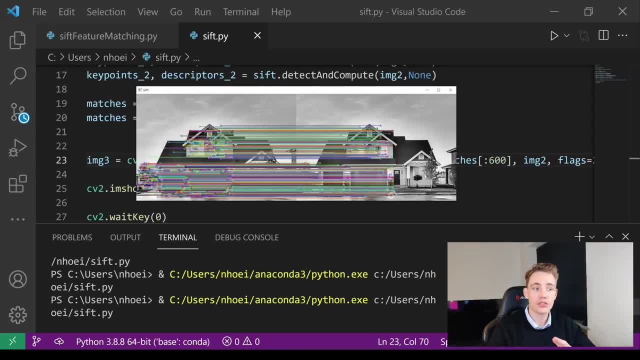 features in the tree here. Now we can't really match points here visually, but we can still see that all the lines here are horizontal. There's no changes from one image to the other, So we're finding the exact same points. but the more points we show here, the harder. 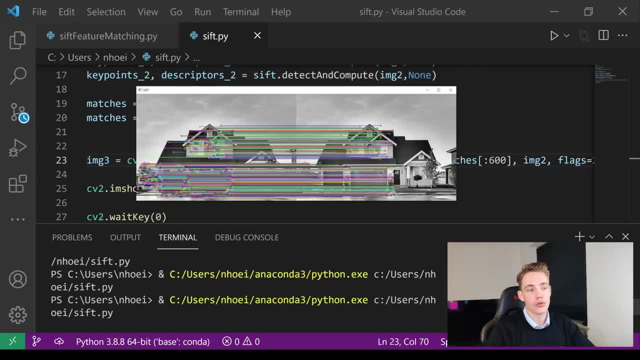 it is. It gets to actually like visualize or like see visually how good are our features actually matching? We can see here in the roof. So this point here is actually exactly at the same point as this one and also all the other points. So we're just finding all the features that we have in our image and then we're matching. 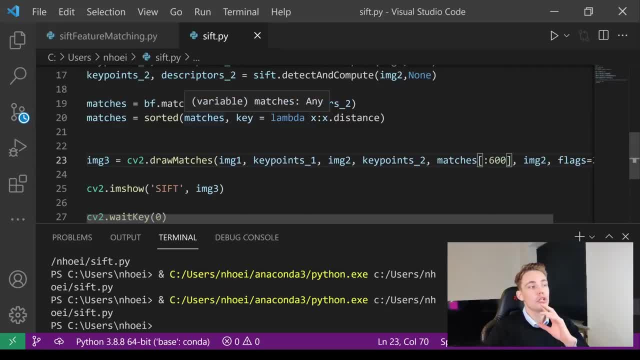 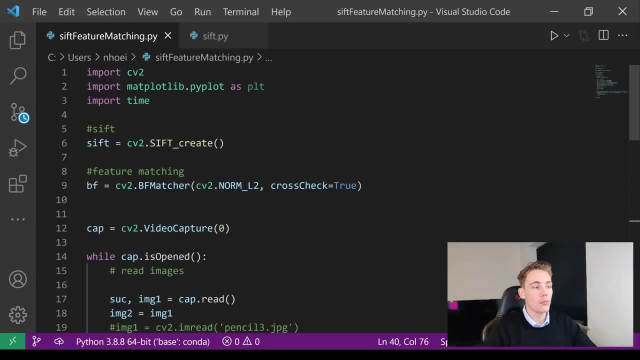 them from one image to the other image. So this is the first script. We're just matching the same image here from one image to the other. Now I'm going to share a script here where we're just going to open up. We're going to do the exact same thing. 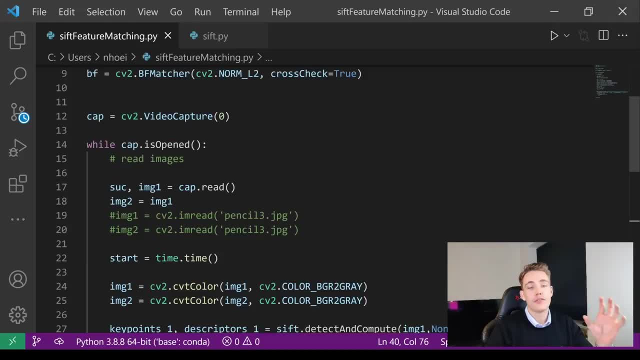 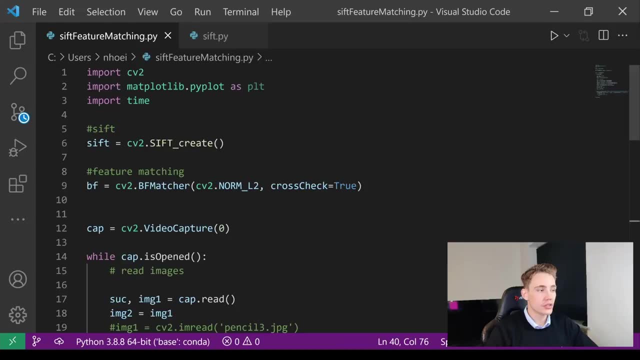 We're just going to open up the webcam feed and then we're going to do SIFT feature extracting on live webcam feed instead of just two images. Again, we're just going to use two images here. So first of all we create our SIFT feature extractor. 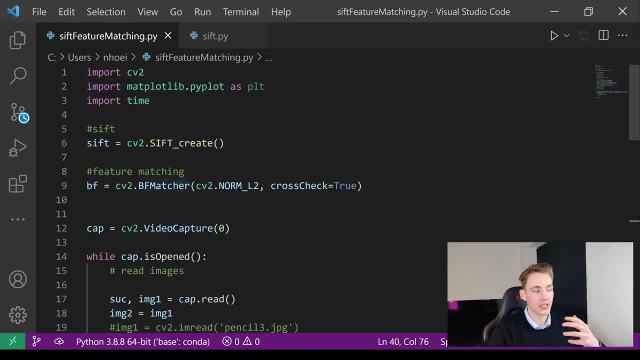 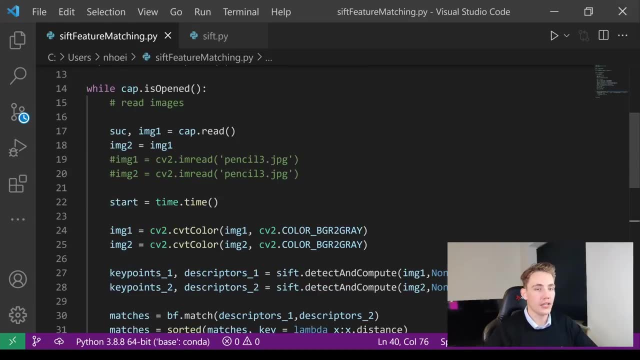 We have our feature matching algorithm or like optics here that we're initializing. So how we're matching the points in the images. Then we're going to open up our webcam. We're just going to have this while running, as long as our webcam is open. 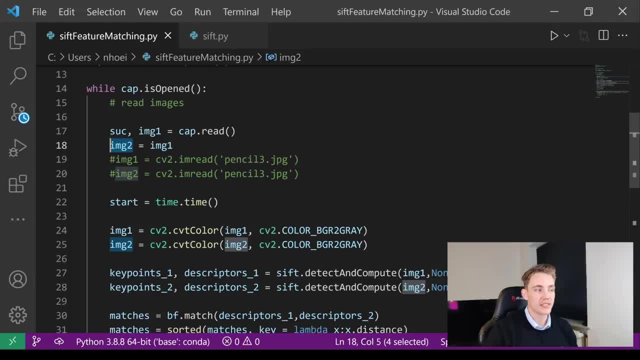 Then we can go down here, read in the first image. Then we're just going to set the second image equal to the first image. So again, we're just mapping points from one image to the other image And then we're finding the exact same points. 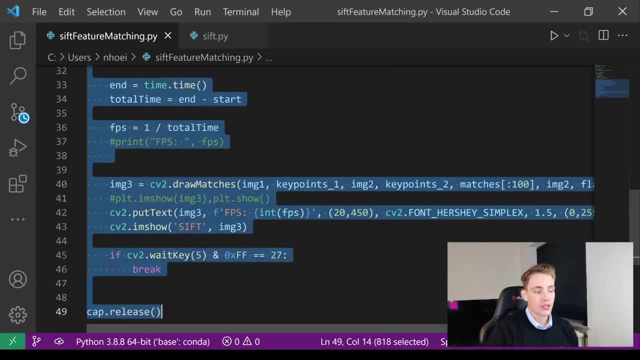 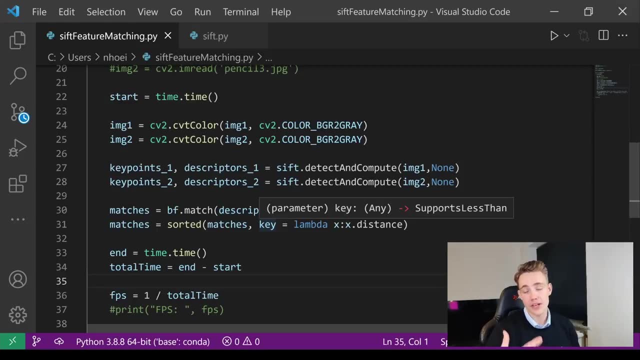 So again, this can be used for stereo vision. All these things here are exactly the same. Right now we just have a timer so we can actually time how fast this algorithm here runs, and how many frames per seconds do we actually get when we're using this SIFT feature extractor? 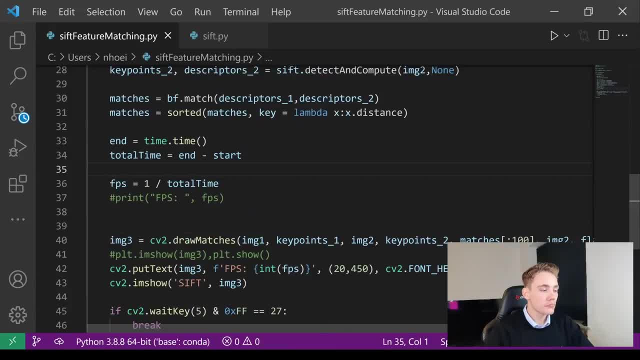 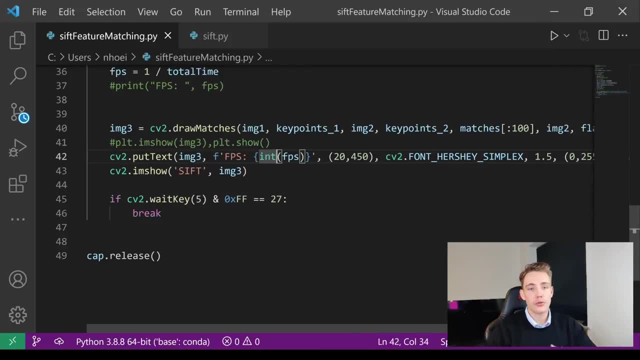 on two images coming in live from the webcam. We're just throwing out the matches. We're just putting out, or like printing out, the number of frames per second that we get If we hit Q or escape on a keyboard at any time. we'll just relieve the webcam or like terminate the program. 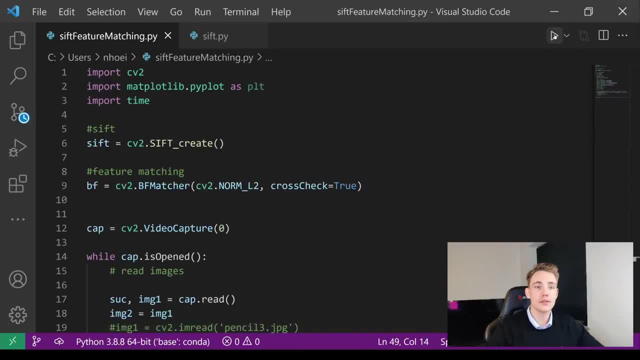 And then we're going to release the webcam. So exactly the same code Again. all the code here that you've seen will be on my GitHub. I'll link to it down in the description here. You can just go into computer vision repository, find all the code here. run it yourself. 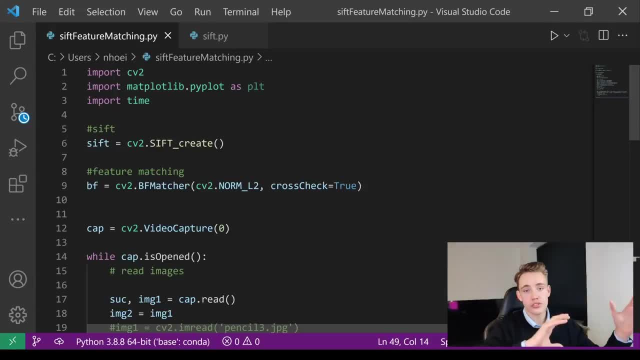 Try to play around with it. Create your own images, Actually try to rotate the images around. Try to see if you can find matches When the object is actually rotated around from one image to the other, and so on. You can also open up your webcam and just try to script out. 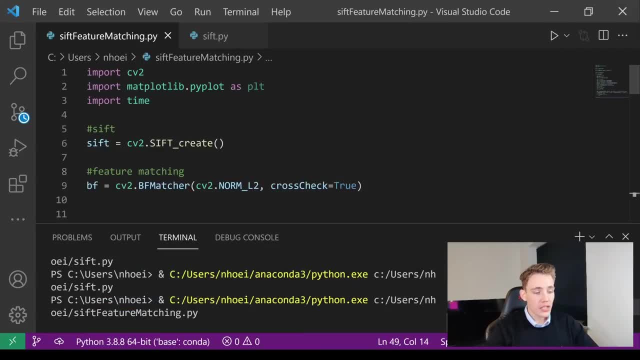 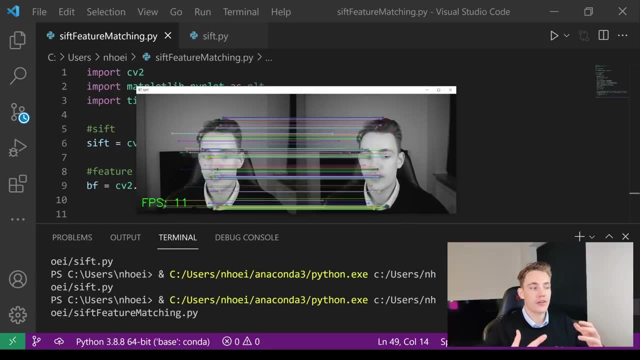 So now we're just going to run a program here, It will open up the webcam. Now we can see that we get up this live video feed here. from the webcam We see we get around 10, 11 frames per second when we're actually running this algorithm. 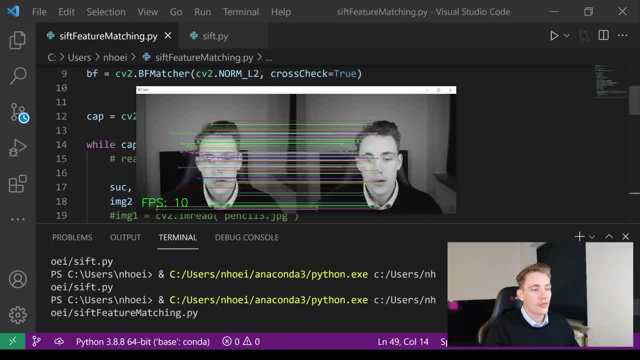 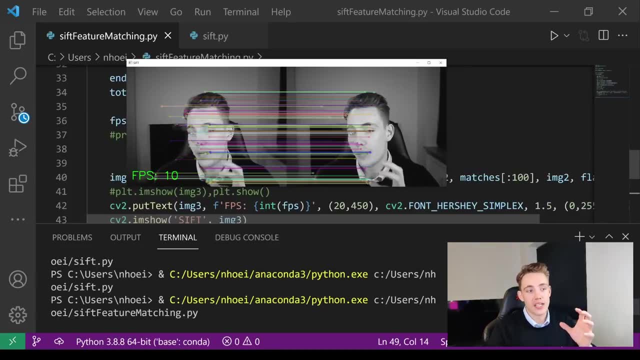 and also displaying all these points here that we're matching right now. If I'm just closing the program, or like at least just scrolling down to the bottom, we only showing 100 matches in our images, So we can actually see what is going on. 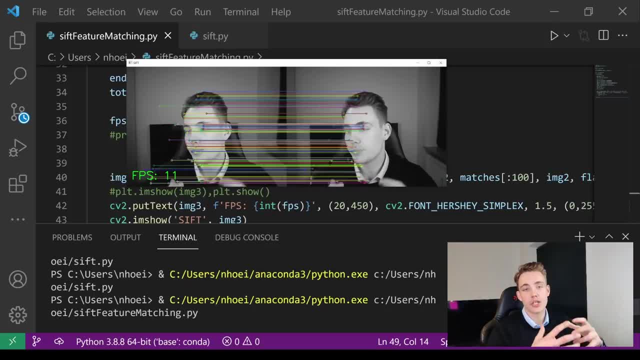 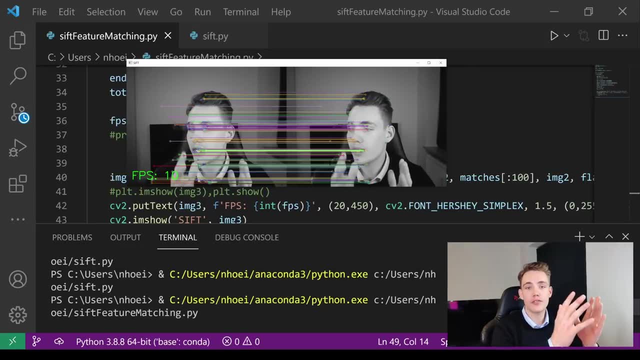 But here we see it is jumping around a lot. This is actually just because we're changing color or like the color. It just shows them randomly from one frame to another frame. So again we're just reading in a frame doing all the process, or like we're just running. 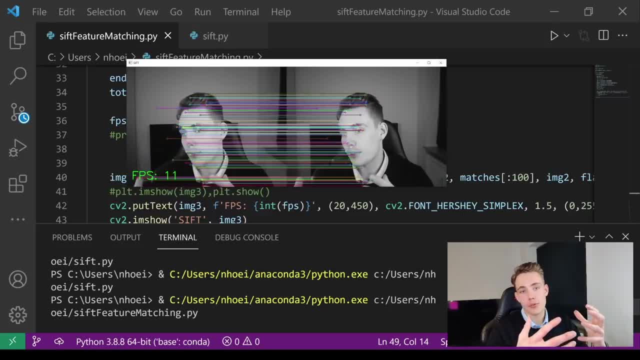 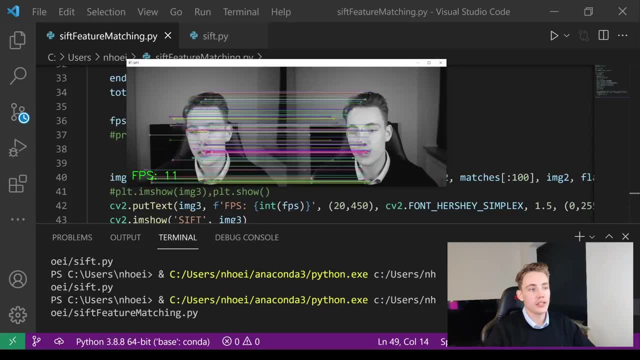 the algorithm on it. Then we get in a new frame, repeat the same process over and over again. So that's why the points here- or like the colors here, are actually flickering. But we see, if I'm holding my head still here, all the lines here. 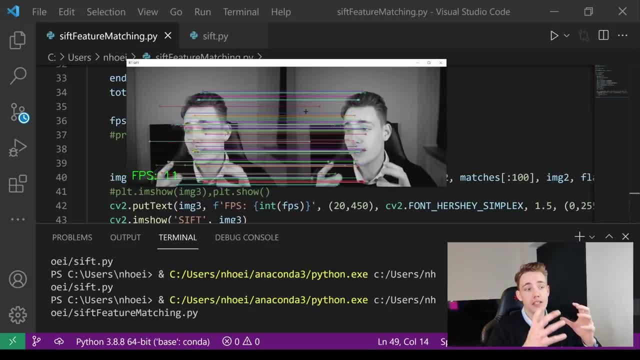 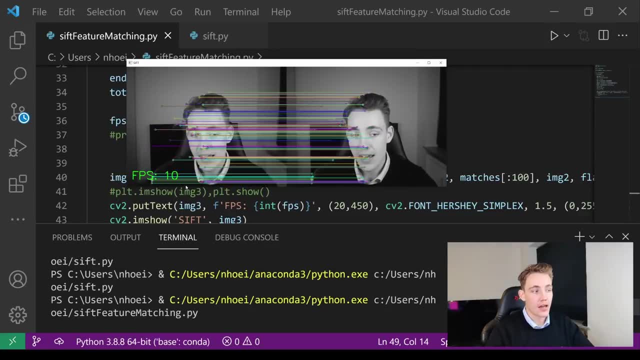 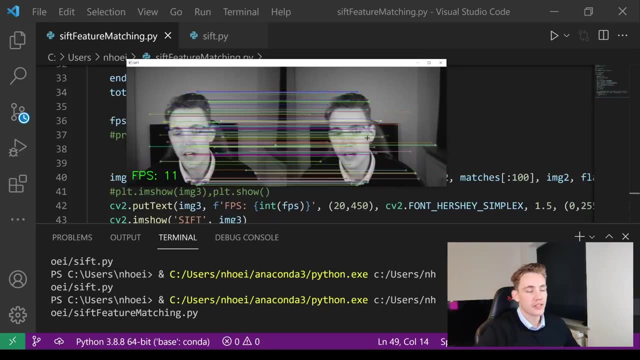 It's actually like the same. It's just changing colors because it is finding the images, or like it's finding the exact same features. every time it loads in a new image from the webcam, which is actually like 10 images per second. If I'm moving around here in the image frame we can see it still finds the different kind. 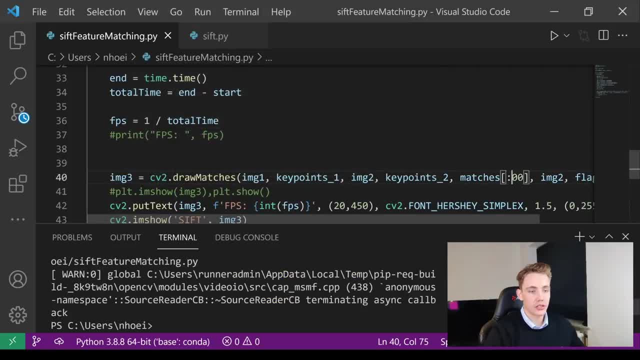 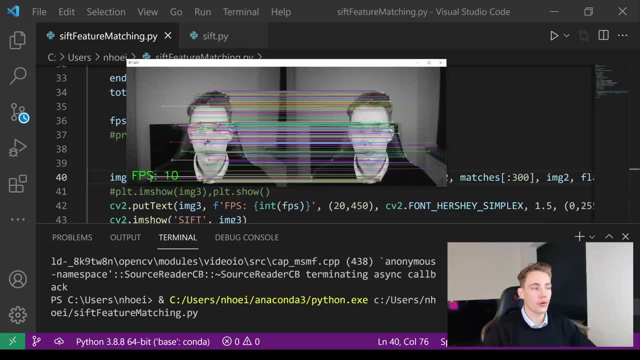 of features. We can try to display a couple more features here. Let's go for, like, for example, 300 and see if we can get some more points. So again here we see. we get a lot more points with my notes. 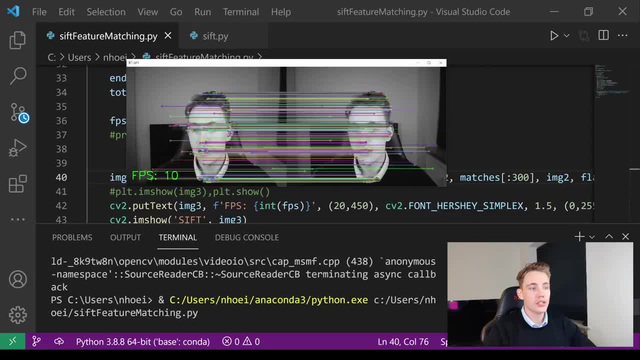 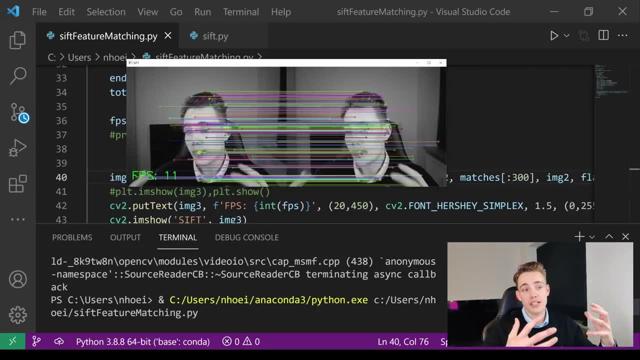 We can see. it is actually like detecting all the points in my nose, ears, also around the hair and stuff like that. It's not really detecting a lot of corners out here in the background because it can't just like it can't find any features. 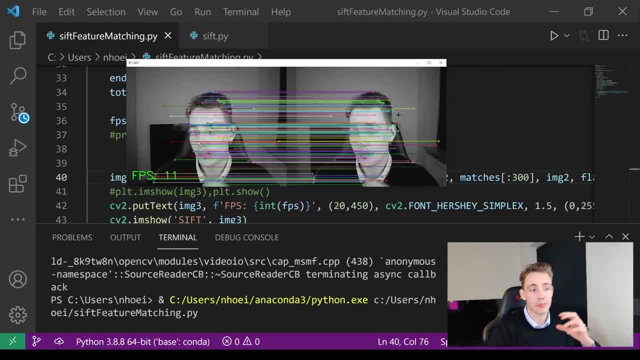 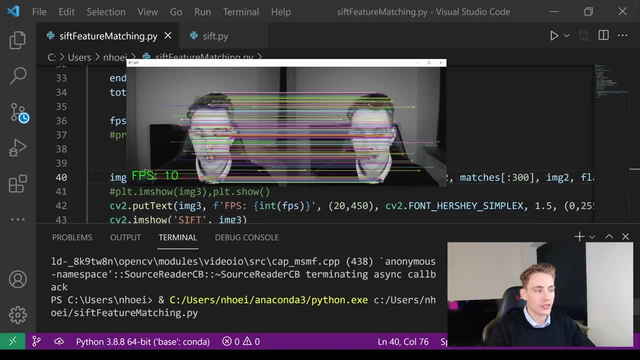 We need some kind of like texture, edges and so on that it can actually match from one image to the other. We can see we get some over here to the right. We get some points over here to the right. We get some here at the shirt. 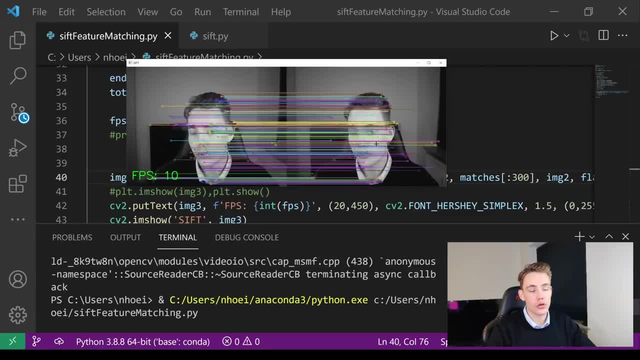 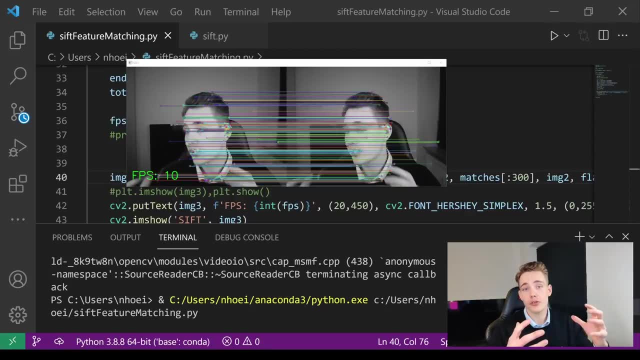 My hair, eyes is really good, Mouth is really good, Nose and ears are also really good. So we can see that we're finding the exact same points from one image to the other image. We're actually going to create a lot of projects where we're going to use this SIFT feature. 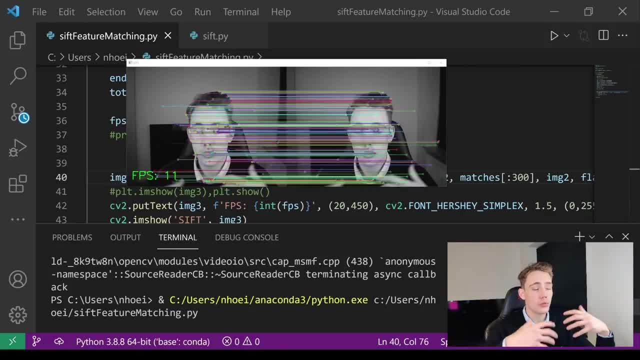 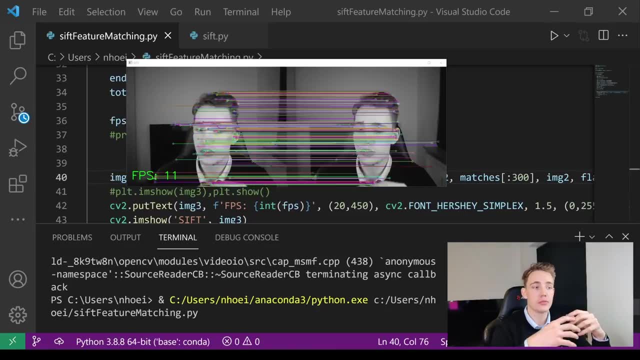 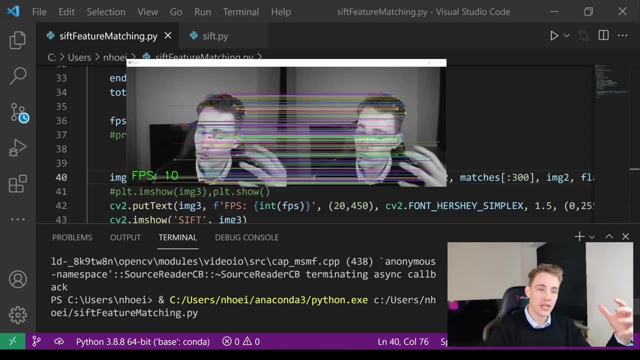 extractor to find points in one image to the other image. So we can actually like do optic detection, finding depth to different kind of optics in the image frame, even like doing post estimation, because we can use like 3D information about all the points when we're using stereo vision to do post estimation, creating point clouds. 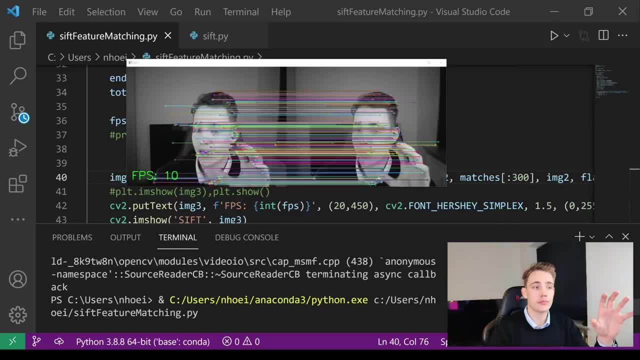 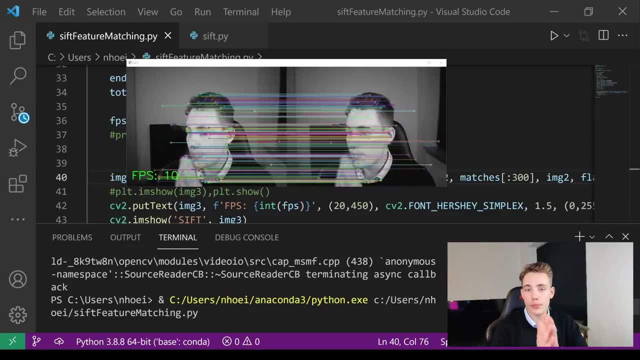 and just like using sparse stereo vision. So we just get some points. Try to find the 3D position of that object or like those points in the actual scene. So remember to hit the subscribe button under the video here and also hit the bell notification. 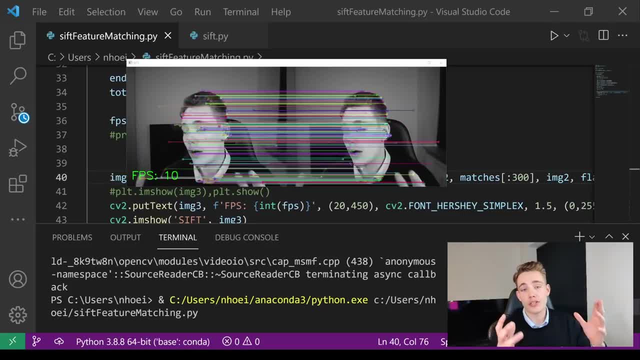 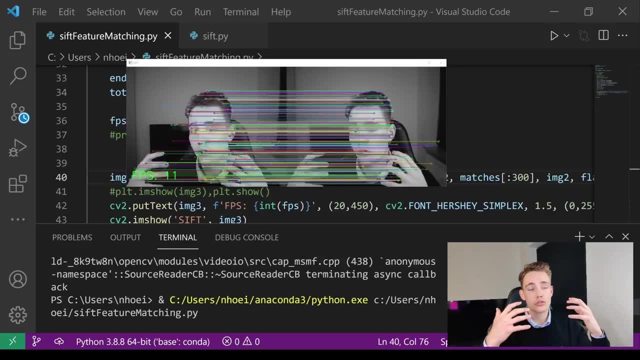 so we'll get a notification when I upload videos about that or in the computer vision tutorial, deep learning tutorial, point cloud tutorial and so on. So thank you, guys, for watching this video here and also remember to hit the like button under the video here. 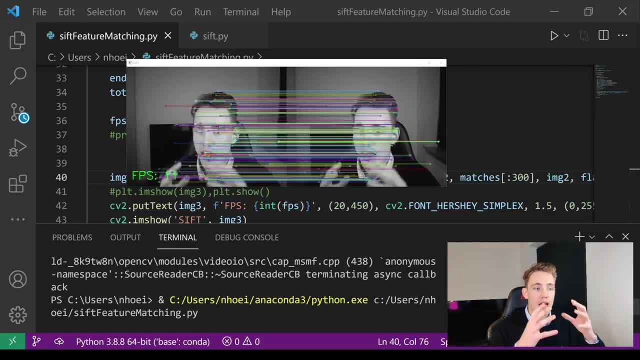 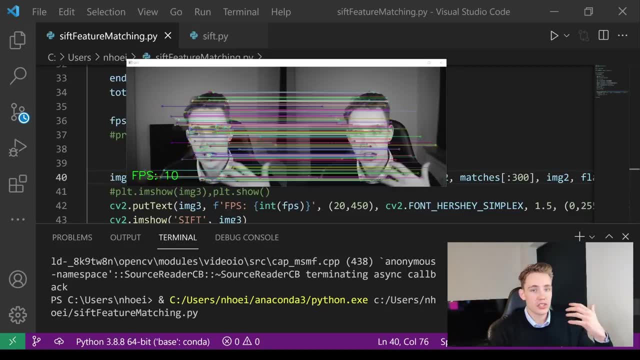 Just really helps me and your channel out in a massive way and I just really appreciate the support. I'm currently just doing this Computer vision tutorial that I've talked about, where we're doing basic image operations, stereo vision, camera calibration and so on. 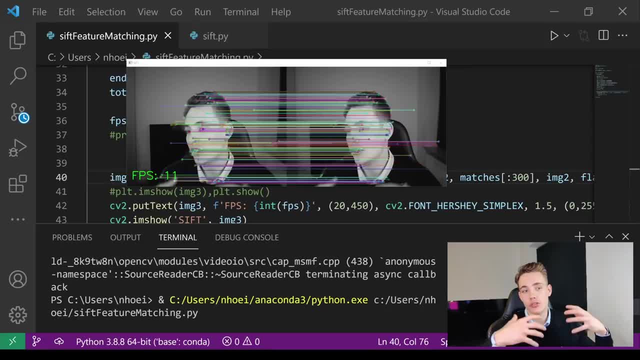 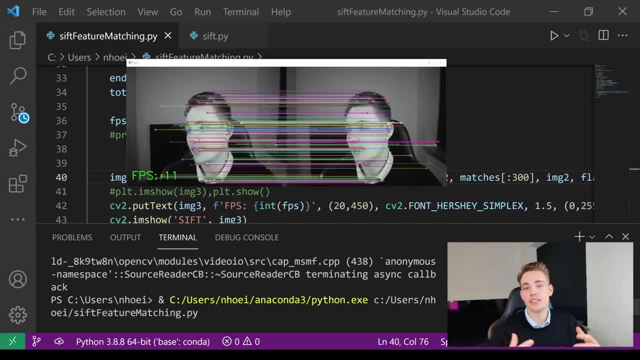 And now we're actually just combining some like all these things here into like bigger projects. We're trying to optimize some of the things and actually create some real life or like some real applications that we can actually use for something. So if you're interested in that tutorial, I'll link to it up here, or else I'm gonna. 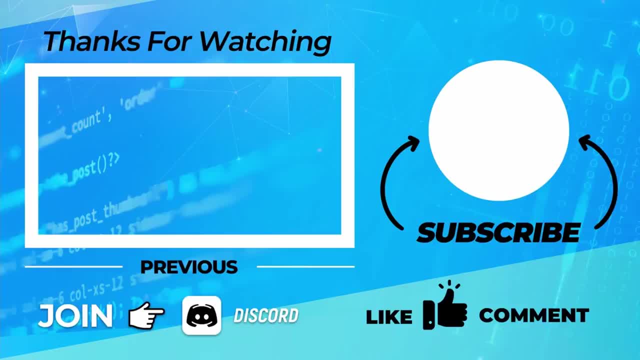 see you next with you guys. Bye for now, Bye.